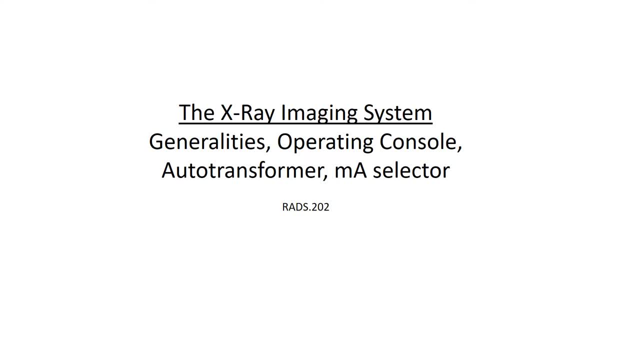 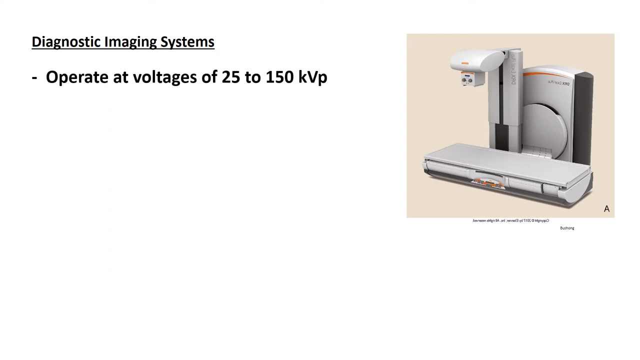 Hello everyone. today we're going to talk about the x-ray imaging system. We're going to talk about the generalities of the system itself, the operating console, the auto transformer and the MA selector Diagnostic imaging systems. they all operate at voltages between 25 to 150. 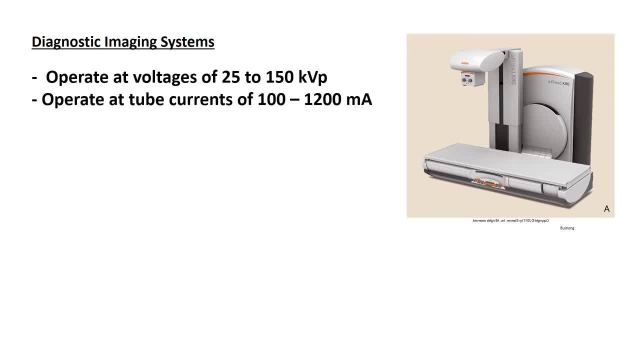 kVp and at tube currents of 100 to 1200 ma. Those are very important facts for you to memorize, especially when you're going to be studying for the registry. So 12 to 150 kVp, 100 to 1200 ma. 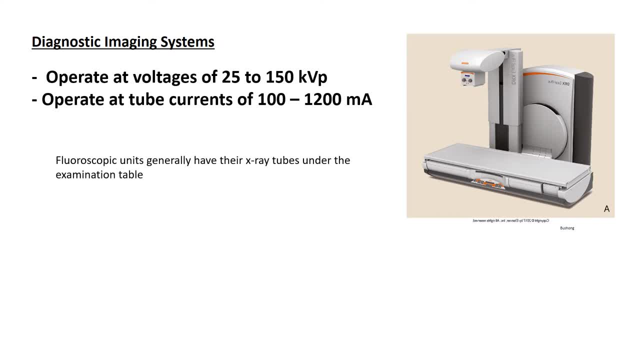 Fluoroscopic units generally have their x-ray tubes under the examination table. We can also call the examination table the couch, and this table, as you know, may either be flat or it could be curved. We can also call it the couch, and this table, as you know, may either be flat or it could be curved. 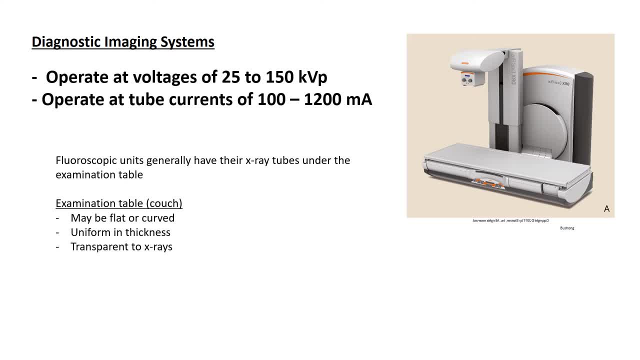 It must be uniform in thickness, as transparent as possible to x-rays, and the material of choice today is carbon fiber. Carbon fiber: it's lightweight but it's very strong, And most of the tables today are floating. They're easily locked or unlocked. Fluoroscopic table or couches are identified. 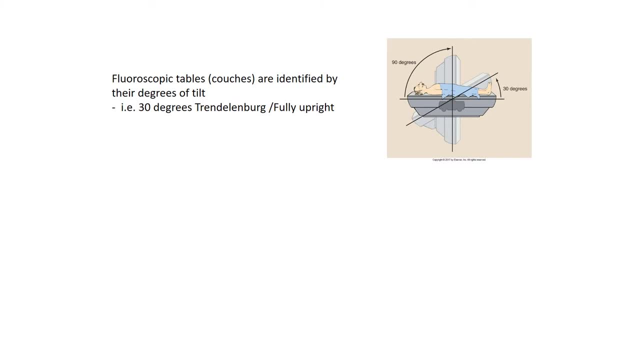 by their degrees of tilt. For example, we could have a 30-90 table. What that means is that the table would tilt downwards 30 degrees in the Trendelenburg position, come up to a full upright vertical position, which would be your 90 degrees. Every x-ray imaging system has three parts. 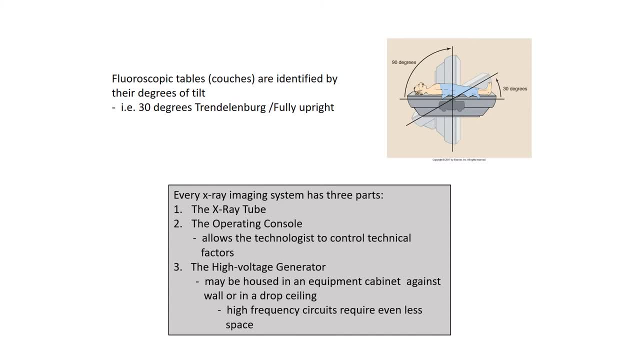 We have the x-ray tube, the operating console, which is where you stand. It allows the technologist to control technical factors, and the high voltage generator, which could be housed in an equipment cabinet against a wall or in a drop ceiling Most of the time today, because 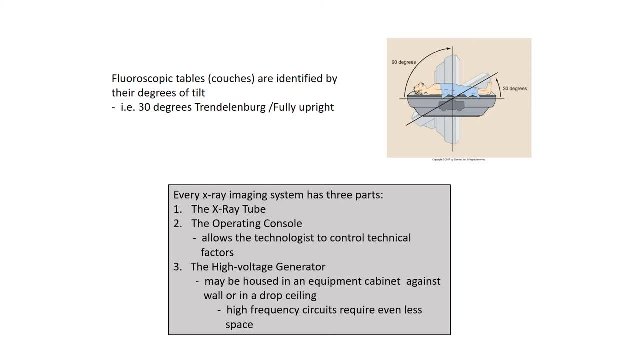 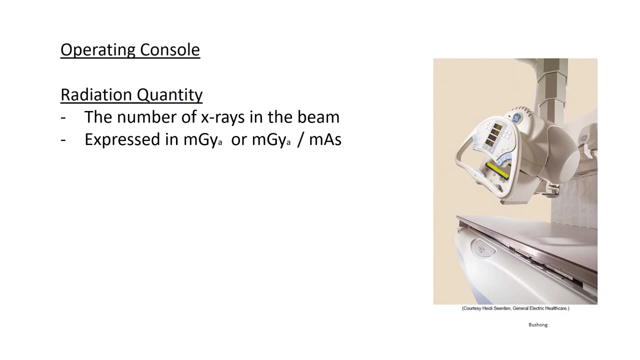 we use high frequency circuitry. it's a lot smaller. It takes up less space. We could put it up into the drop ceiling. It gives you more room in the x-ray room itself. As far as the operating console radiation quantity is the number of x-rays in the beam. It's either expressed in: 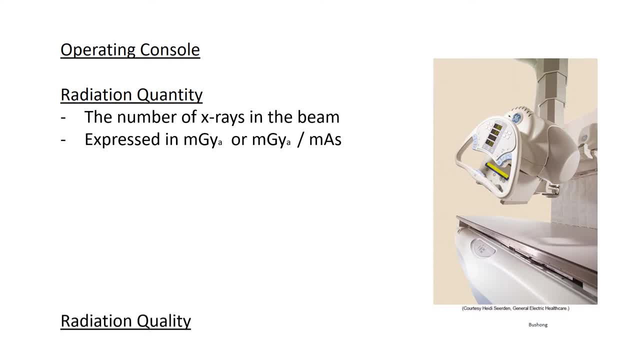 milligray or in milligray per mass. Radiation quality is the energy of the x-ray beam. It's expressed KVP or in half value, layer, HVL, And the console where you stand at provides for control of what's called line voltage compensation, which we're going to talk about today: KVP, MA and exposure time. 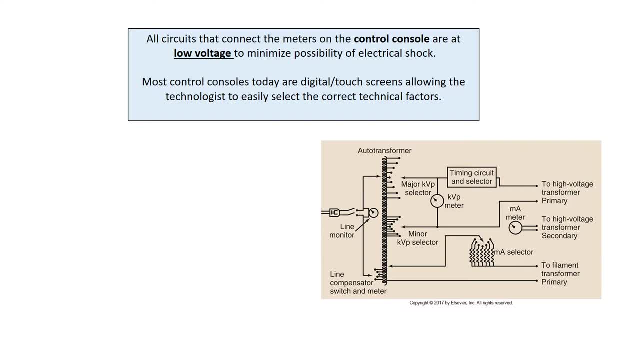 All circuits that connect the meters on the control console are at low voltage to minimize the possibility of electrical shock. Now, this is going to be important for you to remember that everything on your control console has to be at low voltage When we begin looking as we. 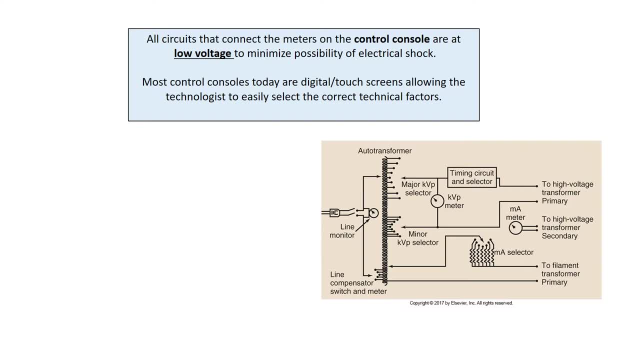 are today at the x-ray circuit, we're going to notice that there's a high voltage portion and a low voltage portion. Most control consoles today are digital or touch screens, which allow the technologist to easily select the correct technical factors. In fact, 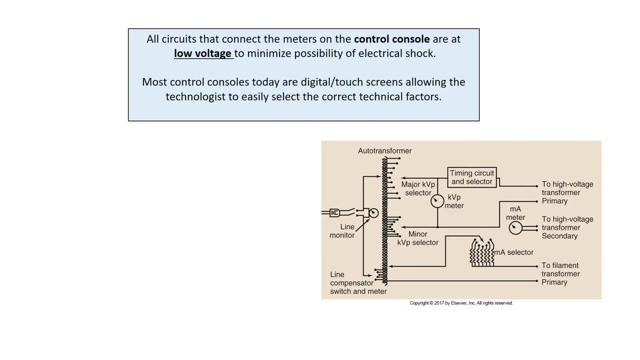 most of your equipment today. you're going to do a hand, an abdomen, whatever. you simply click on it and it sets all of all of the technical factors up for you. Now I want you to look to the drawing at the right. This is a part of the x-ray circuit I want you to notice on the left-hand side. 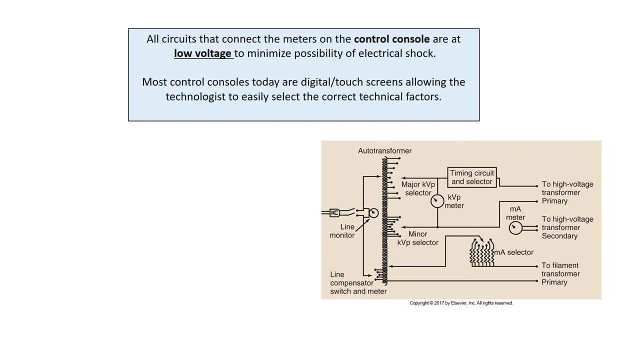 where it says line monitor, it looks like a plug is coming in. This is representing the incoming power source that we're going to get from the electric company, Now the first thing that that electricity is going to go into as far as the circuit is concerned. 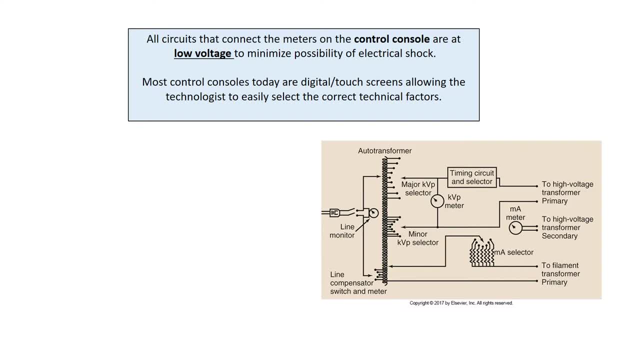 is called an auto transformer. I'd like you to look down at the bottom of that auto transformer and notice it says line compensator. Sometimes it's called a line voltage transformer, Sometimes we'll just say line compensator, switch and meter. What's important is that most systems today are designed to operate on 220 volts of power. 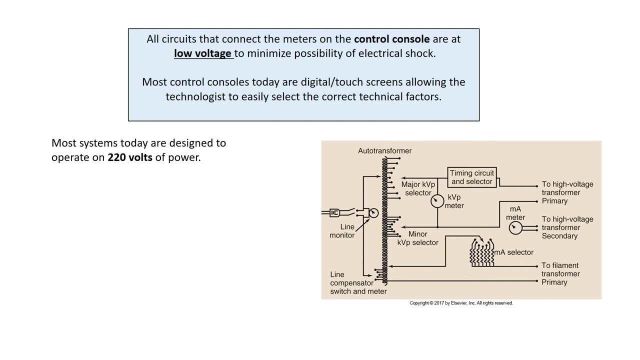 So we have power being generated- 110 volts, 60 cycles- by the power company. of course, if we take two 110 lines, we end up getting our 220 volts of power, And that's the amount of power that's going. It's important to understand that from the power company we are getting volts, but to take an x-ray we need kilovoltage, thousands of volts. 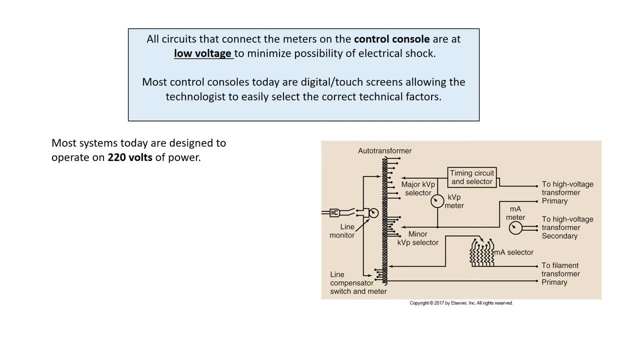 So there's going to be things within the circuit that are going to be able to take that voltage from 220 and bring it up to the level that you're going to need to take an x-ray. For example, you're taking a chest x-ray, you might need 120 kVp. 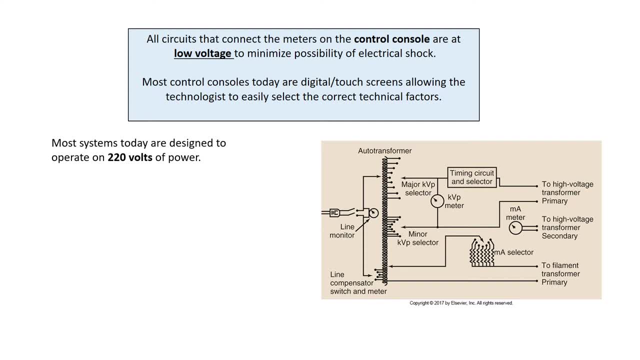 If you think about it, that's 120,000 volts of electricity that we're going to need Now. unfortunately, the power companies cannot deliver exactly 220 volts consistently. Sometimes it goes up to 225, sometimes down to 215.. 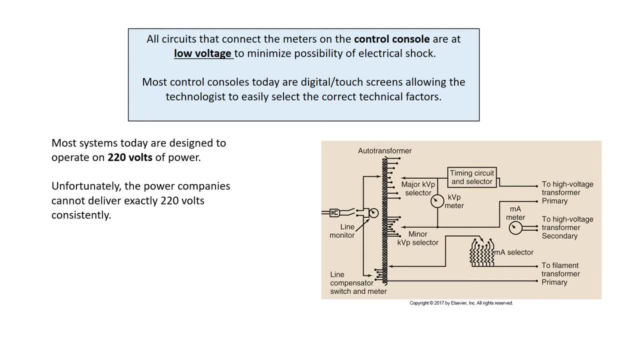 Now most of the appliances in your home. it doesn't matter really that much If we up the voltage or bring the voltage down a little bit, as long as we're around that 220 volts. However, for the x-ray circuit- 220, it needs to be very, very specific. 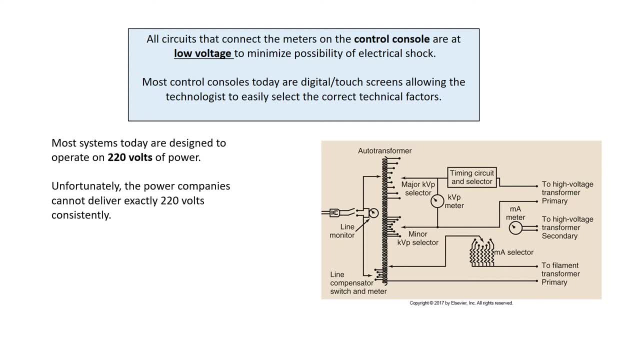 Because what's going to happen is the voltage coming from the power company is eventually going to be fed into what we call the step-up transformer, which is going to bring you to your kilovoltage level. Now there's a formula that we have learned about transformers and we know that when we take the voltage on the secondary side, we compare it to the voltage on the primary side. 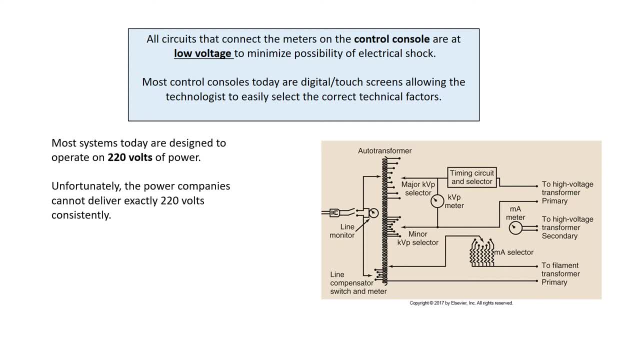 If it's a step-up, the voltage on the secondary side is going to be increased and it's going to be increased to a certain number. The step-up transformer has a fixed number of coils. That's important to remember. The step-up transformer has a fixed number of coils. 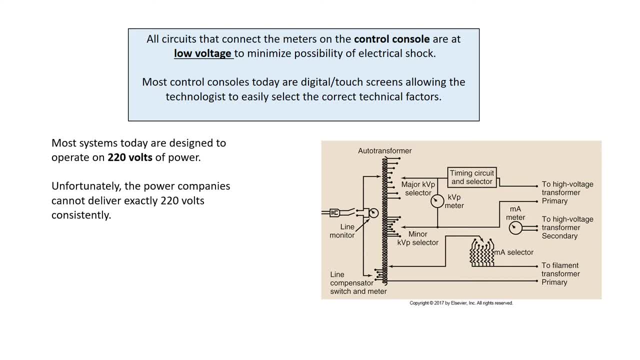 So in order to vary the amount of electricity coming into the step-up transformer, we have to somehow manipulate that voltage of 220 up or down before it gets fed into the step-up transformer. Now the 220 volts coming into the step-up transformer is going to be increased to a certain number of coils. 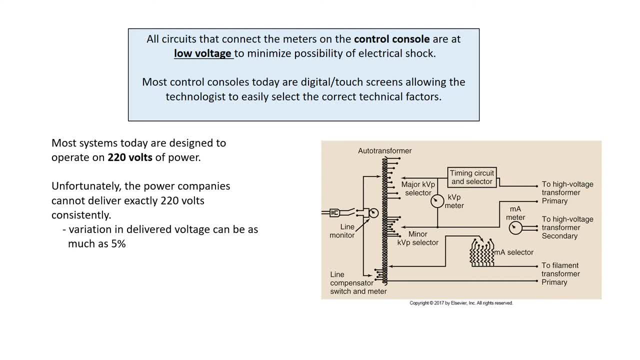 The many volts that come in to the equipment itself, into the circuit from the power company can have a variation by as much as 5%. Once again, we want to be very specific and have exactly that 220 volts, If you didn't. 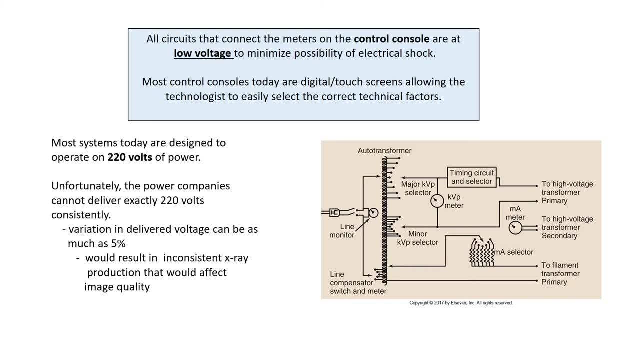 get it to exactly 220 volts and you had this variance, and then you fed that amount of electricity into the step-up transformer, which has a fixed power- containing difficulties. there's no Producer in the power company If you didn't get it to exactly 220 volts and you had this variance and then you fed that amount of electricity into the step-up transformer, which has a fixed amount of driving power. so you should never buy this power container to add to your dirts. 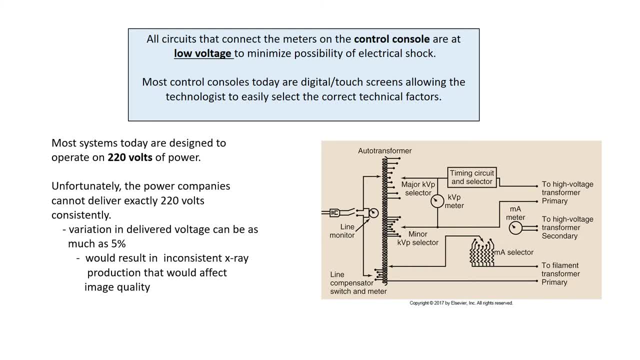 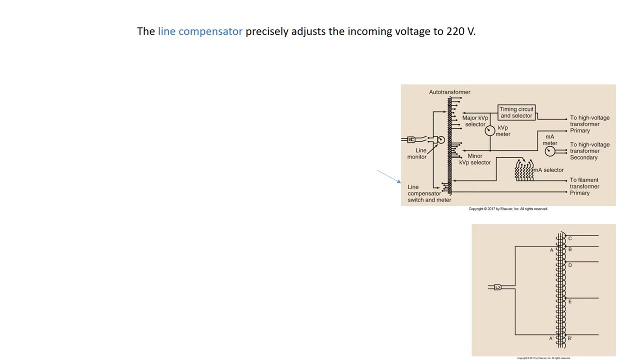 number of coils, you'd get very inconsistent x-ray production and this would certainly then affect the image quality. Down at the bottom on this drawing to the right at the top, you have the line compensator. What this does remember is you have that variance of the 220 volts coming from the power company. 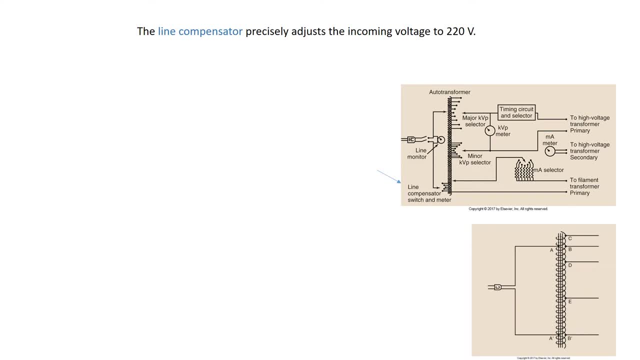 Maybe it's 225.. We've got to get it right back to 220, and that's the job of the line compensator. It adjusts the incoming voltage to exactly 220 volts. Now, on older equipment, you actually had a dial on the controller. 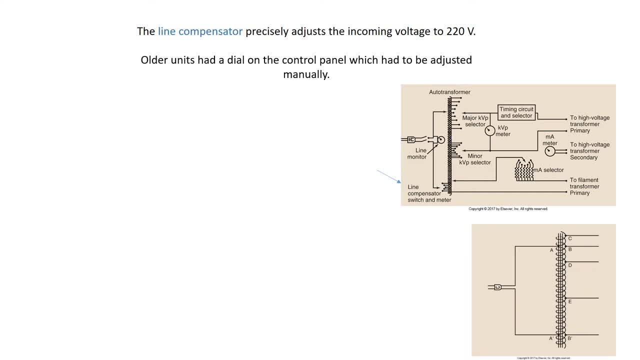 You had a control panel which you had to literally adjust manually. It appeared as a needle, basically, and there was a line right in the middle and there was an arrow. Sometimes the arrow would be to the right or to the left of the middle line. 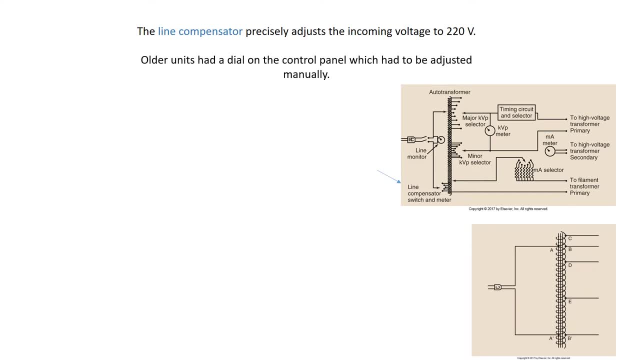 What you had to do as a technologist is, when you came into the room before you made the exposure, you'd have to adjust the control panel. You'd have to adjust the control panel, You'd have to turn a dial. and when you did, that little needle, that little arrow would jump. 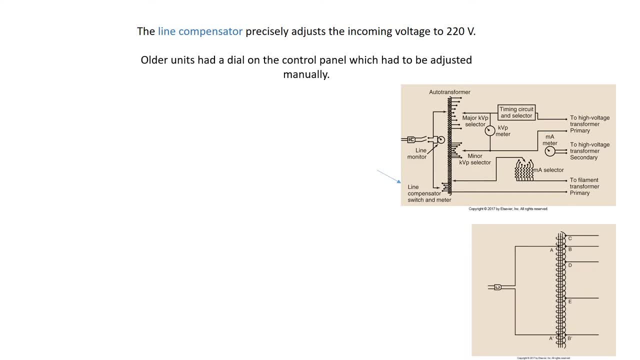 and you would keep turning it until you got that needle right in the middle, right where the middle line was, and that would tell you then that you have now 220 volts. We don't have that anymore on the control panel. It's all done internally, okay. 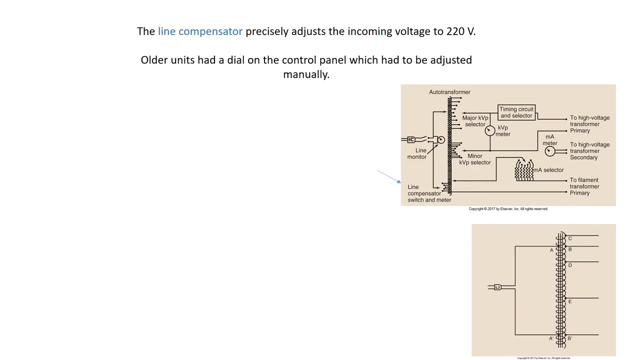 So the line compensator is still there. It's not like it's gone away, Okay, But it's nothing that you, the technologist, will have to manually adjust anymore. It's all done internally by the circuitry itself. The power supplied to the X-ray imaging circuit is delivered first to the autotransformer. 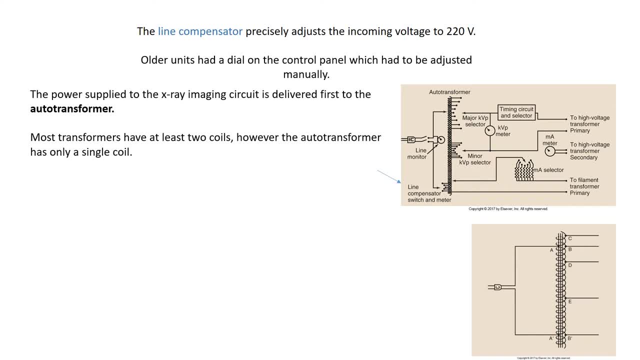 Now, when we think about transformers- we studied them a little bit before. Most of your transformers have at least two coils. However, the autotransformer only has a single coil. This is why we have that prefix: auto. Auto means self. 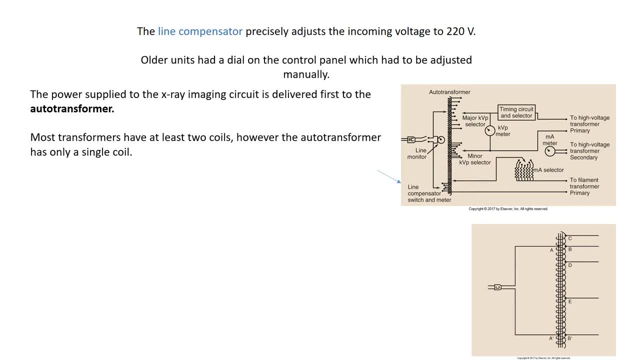 The autotransformer only has a single coil. This single winding is designed to supply a precise voltage to both the filament circuit and to the high voltage circuit. So as we go along, we're going to have to adjust the control panel. 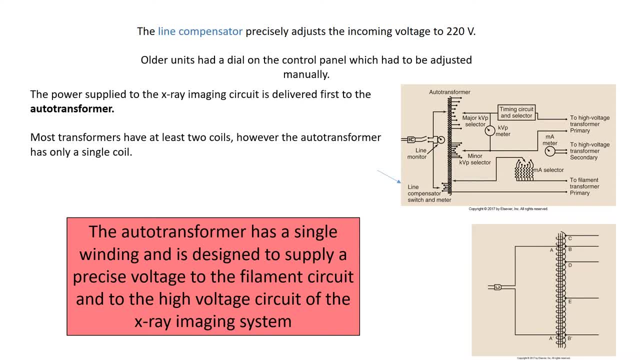 As we continue our study of the circuit, what we're going to see is that one part of the circuit is going to be the high voltage part of the circuit. That's the part of the circuit that's going to have a step-up transformer. 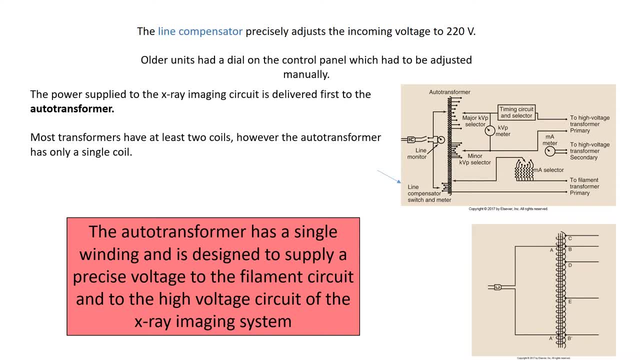 Because when we say step-up, what are we stepping up? We're stepping up the voltage In the other part of the circuit. we need low voltage And we need low voltage to heat up the filament. To heat up the filament, we need low voltage. 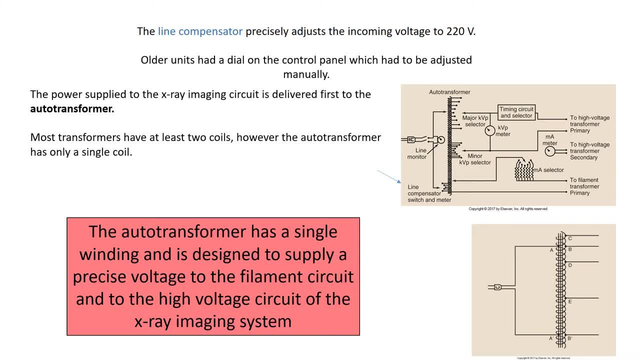 High amperage. So in the filament part of the circuit- this is going to be the low voltage part of the circuit- We're going to need a step-down transformer to take that voltage of 220 and bring it way down. Now, of course, when we bring the voltage down, the amperage goes up. 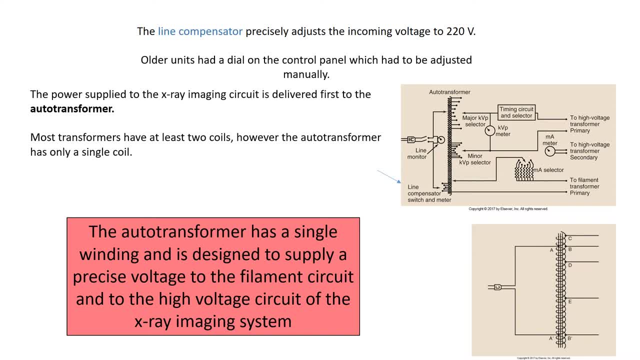 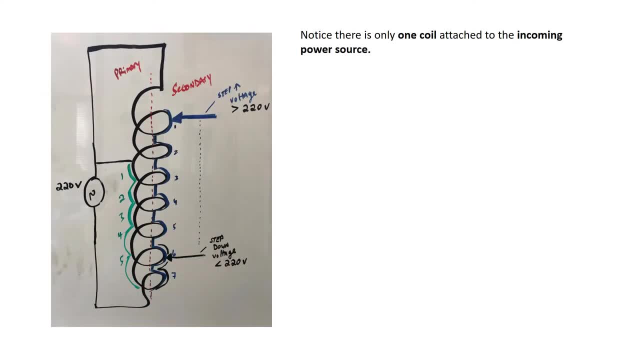 So the autotransformer is responsible for supplying voltage into both parts of the circuit. Over on the drawing on the left, I tried to draw here for you an autotransformer. I'd like you to notice that where it says 220 volts, there's a little symbol which indicates this is alternating current. 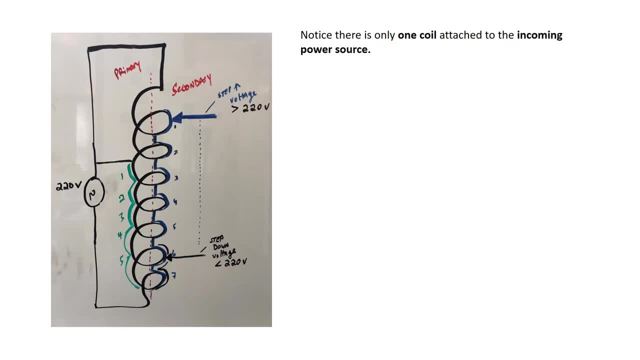 What I'd like you to notice is that you've got a single coil. What I've done is I've drawn a red dash line Down the middle of that coil. You can look at this coil then as having, even though it's just one coil, a primary side, which is on one side of the dashes there in red. 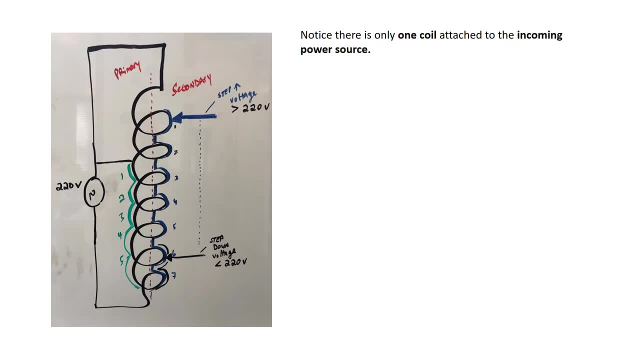 And then one side would be considered the secondary side. The next thing I want you to notice is that I've got a connecting wire at Where it says number one in green. All right, So if we then count the number of coils starting from that connecting wire, we've got one, two, three, four, about five turns of the coil on the primary side. 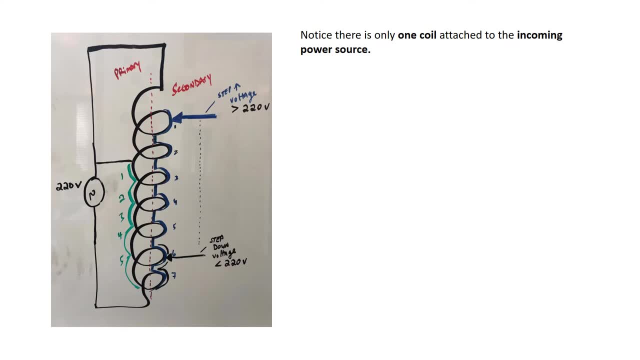 On the secondary side, we've got two arrows drawn. Now. these two arrows are points, Points of contact. We can also call them taps, T-A-P-S. They're points of contact And these points of contact are going to then connect to the rest of the circuitry. 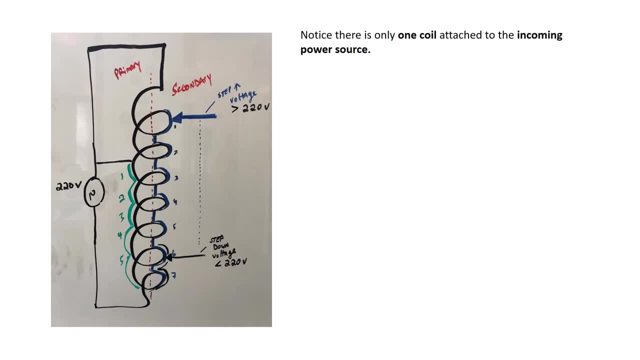 The rest of the electricity that's going to be going into, eventually, the step-up transformer. This arrow, this point of contact, has the ability to move up or to move down. So I have one thicker arrow drawn in position number one And then another arrow, a little thinner arrow, drawn at position which would be six here. 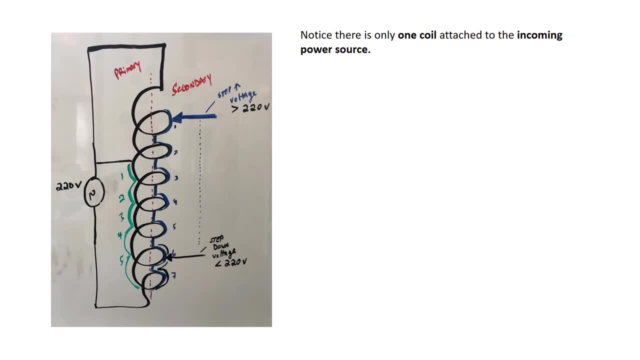 Now that arrow, that point of contact, moves up and down. And it moves up and down when you change your kilovoltage. Now, in older equipment you don't find this really today much, But in older equipment when you would turn a dial and you would go. 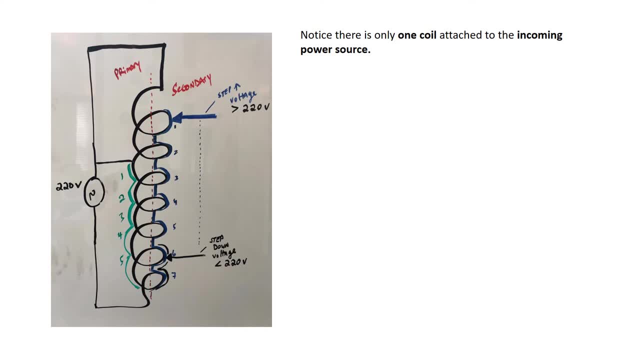 from one kilovoltage to another, it would make a very unique sound. It kind of sounded like this, And basically what that was is the point of contact, either moving up or down on the auto-transformer. If we look at this auto-transformer, let's look at the thick arrow. 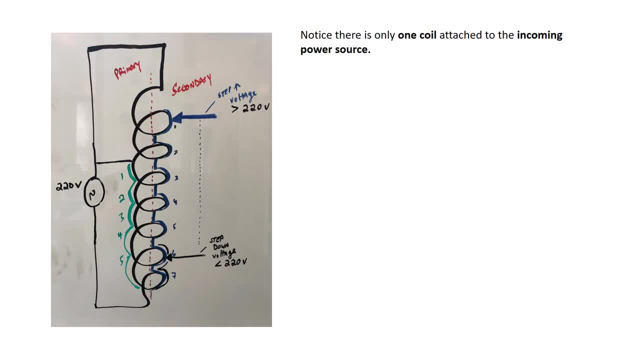 And remember, I'm looking at the one coil And I'm looking on the right-hand side. So when we have the thicker arrow, position number one, I've got one, two, three, four, five, six, seven coils tapped off. 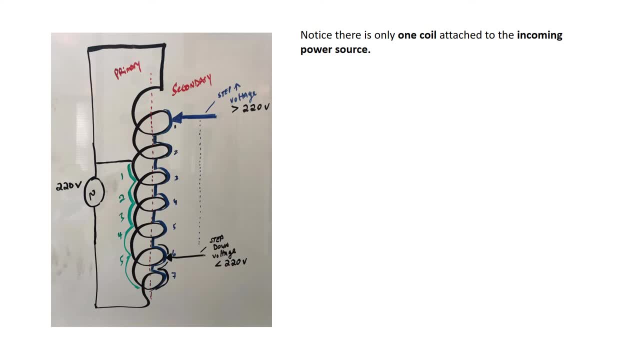 Now, if I look on the other side of the coil, the primary side, I only have five coils tapped off. So when I look at this- five coils on the primary, seven coils on the secondary- What's going to happen now is I'm going to step up the voltage. 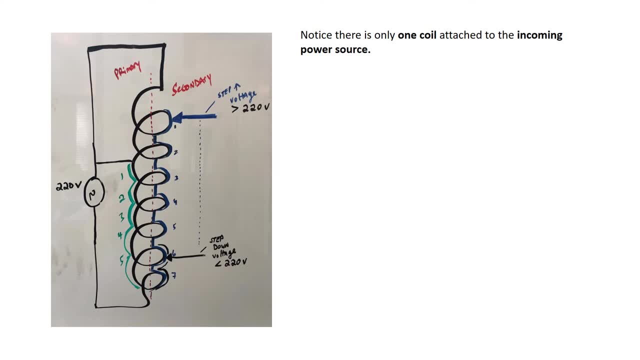 I'm going to be utilizing all of the coils on that side: One, two, three, four, five, six, seven. So it's five to seven. I'm going to step up the voltage If we look at the thinner arrow. well now, on that secondary side, I've only tapped off two coils. 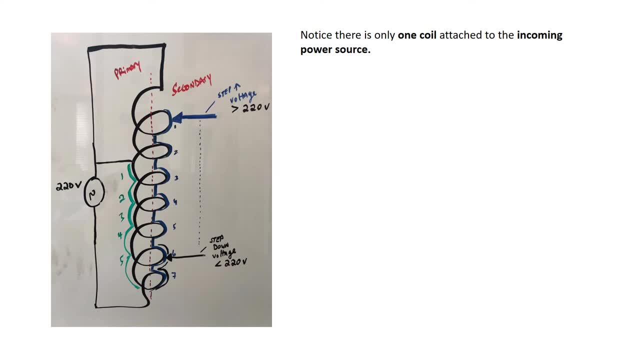 This would be six and seven. So now I've got five coils on the left-hand side, the primary. Now only two coils I'm tapping off on the secondary. So what am I going to do? I'm going to bring the voltage down. 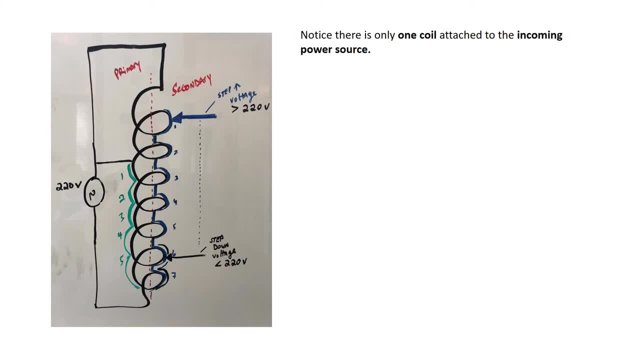 So in position one where I've used all of the coils on that side, I'm bringing the voltage up When I bring it all the way down and I'm only tapping off two coils on the secondary side. well, now I'm going to bring the voltage down. 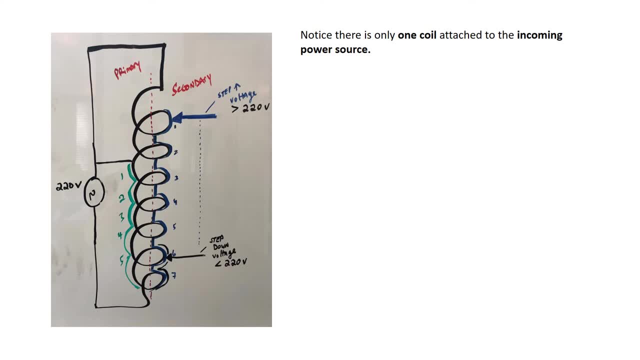 Now I've only got seven coils drawn here. Of course, in actuality there's hundreds of turns, if not thousands of turns, on this auto-transformer of the coil, But here I just wanted to do it simplistically to show you. 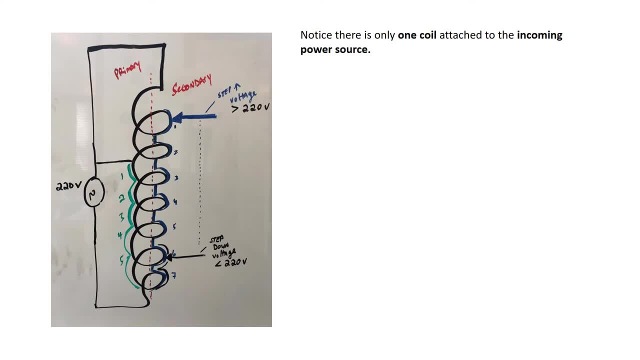 When you tap off more on the secondary side, you're going to step up the voltage. When you tap off less on the secondary side, you're going to step down the voltage. So, as I said, think of one side of the coil as being the primary side, the other side of the coil as the secondary side. 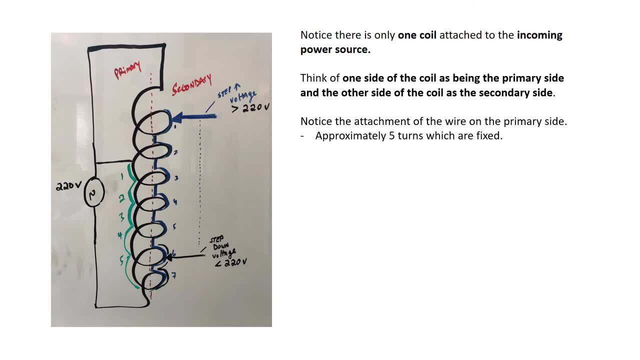 Notice the attachment of the wire. on the primary side approximately five turns which are fixed. The arrows on the secondary side represent a movable point of attachment. If it's in the blue position, there are more turns on the secondary than on the primary side, so seven compared to the primary having five. 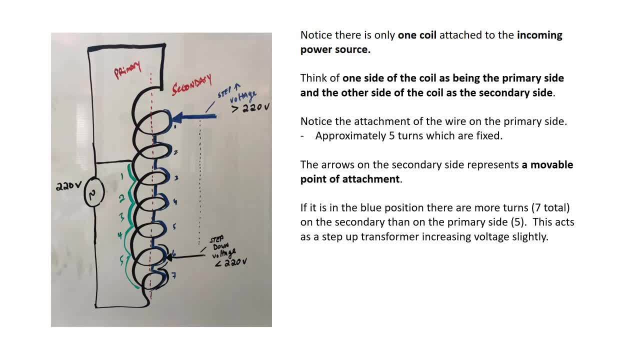 As I said, this would act as a step-up transformer, increasing the voltage slightly, And if it's in the black position down at the bottom, there are less turns on the secondary. only two turns now tapped off, But five still remain on the primary side. 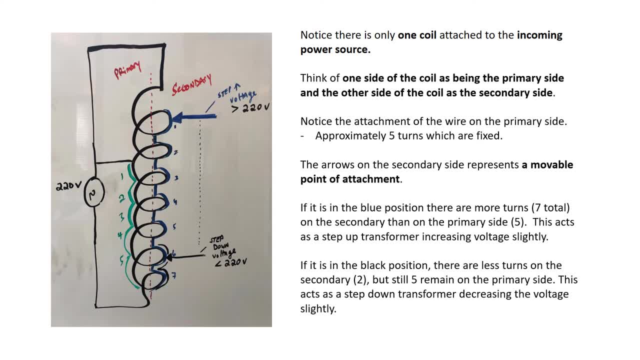 This acts as a step-down. This is a step-down transformer decreasing the voltage slightly, So I hope that makes sense. Remember, on the secondary side, a movable point of contact either allowing you to tap off more or less coils. 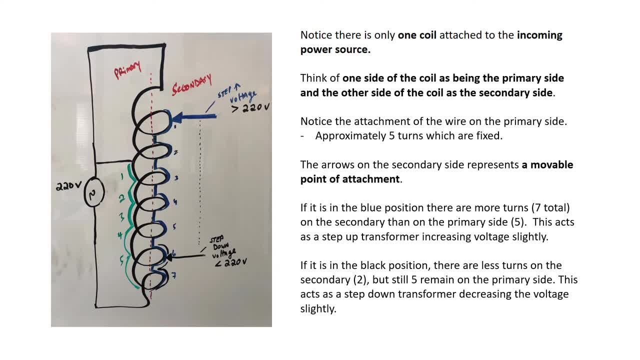 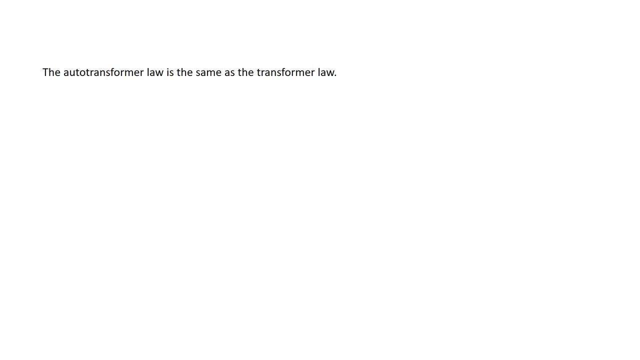 The primary side is going to have a fixed number. This is going to allow you to change that incoming voltage. The auto-transformer law: it's the same as the transformer law that we've learned, So you could calculate the voltage on the primary side of the auto-transformer. calculate the voltage on the secondary side of the auto-transformer. 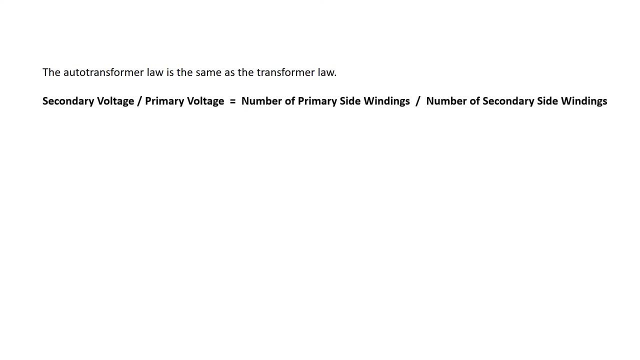 Remember the formula is: secondary voltage divided by primary voltage equals number of primary side windings divided by number of secondary side windings. So on the registry on an exam you may get an example like this: If the auto-transformer is supplied with 220 volts to the 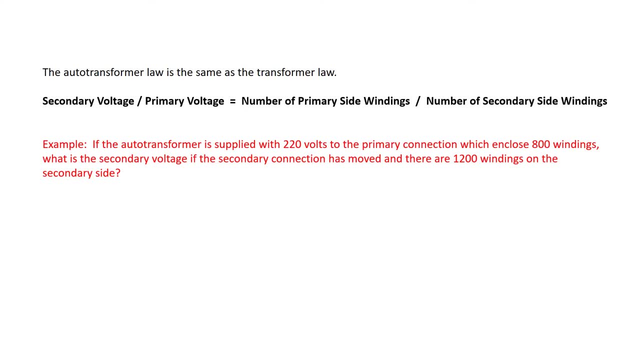 If the auto-transformer is supplied with 220 volts to the primary connection, which includes 800 windings, what is the secondary voltage if the secondary connection has moved and there are now 1,200 windings on the secondary side? So you think to yourself before you even do any math, and this is what I always tell students. 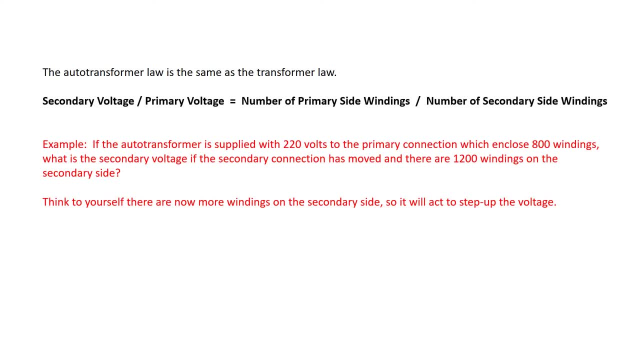 think to yourself: am I doing the math involving a step-up transformer? Well, if I am, my answer in voltage better be going up If it's a step-down. If it's a step-down transformer, my answer should be less. 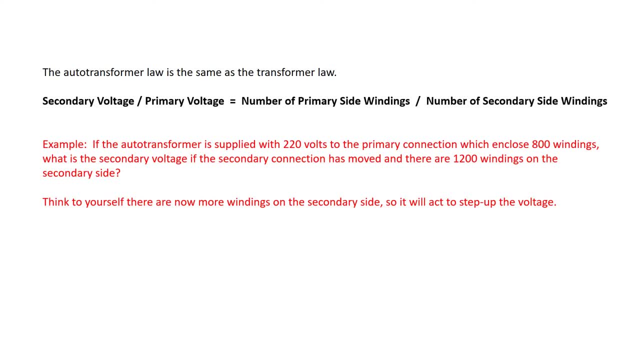 So, as it says here, think to yourself. there are now more windings on the secondary side, so it will act to step up the voltage. So when we do the math, it would be X, number of volts divided by the 220 volts which is on the primary side. 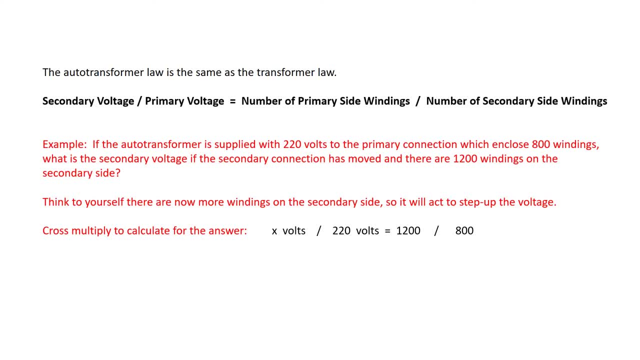 equaling 1,200 divided by 800.. We're going to cross, multiply To calculate for our answer. so we're going to end up with 264,000 equaling 800X. Our answer then would be 330 volts. 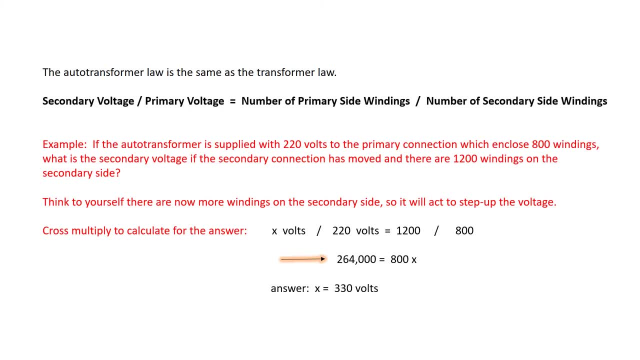 So we've gone from now 220 and we've stepped it up to 330 volts. This now is the number of volts that is going to be fed into the step-up transformer. That 330 volts is going to be on the primary side. 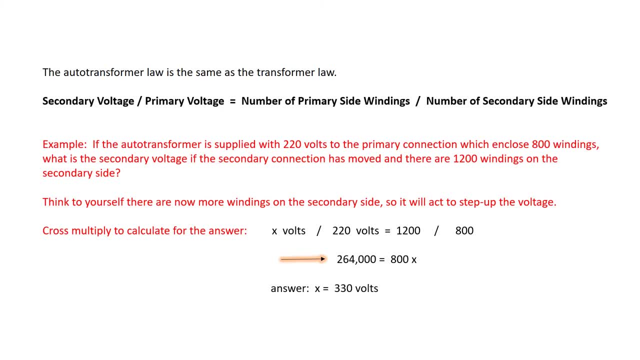 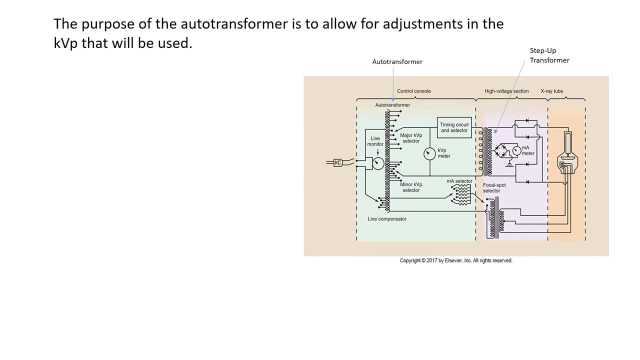 Now, depending on the number of coils on the step-up transformer, we're going to bring up the voltage from that point. So the purpose of the auto transformer is to allow for adjustments in the KVP that will be used. I want you to look at the drawing. 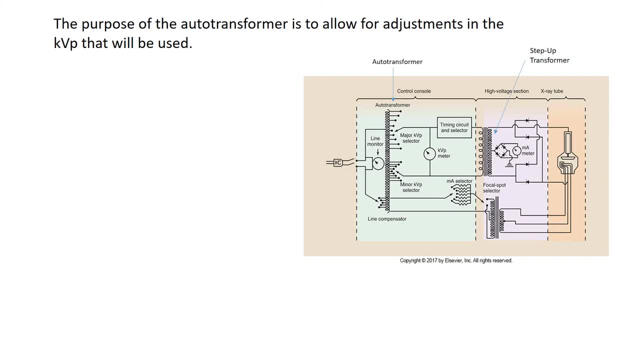 So we've covered so far the incoming power source, which is at the far left. It's not identified, but this would be there. It looks almost like a plug coming in indicating this is the incoming power source. Now, this is the auto transformer. 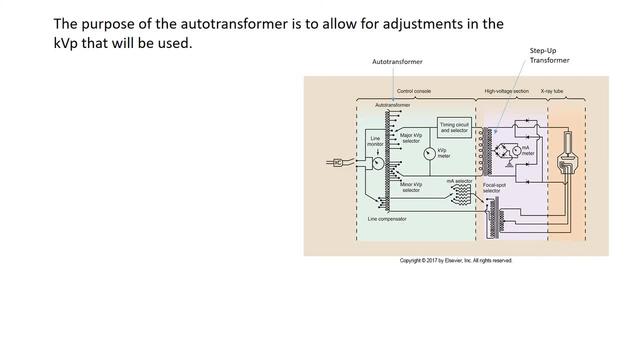 This is the power source source. We said that we need to get it exactly to 220 volts before we do anything, so that's the job of the line compensator, or line voltage compensator. You can see you've got the auto transformer. Remember, the auto transformer is going to take now the 220 volts that we're getting. 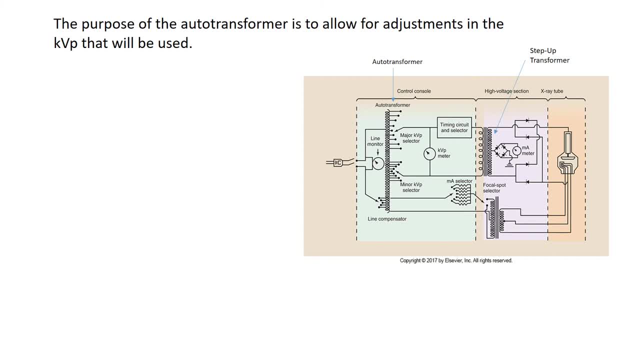 from the power company and it's going to bring it up. We're going to bring it down and then we're going to feed the electricity. If you follow over to the right on the top, eventually it's going to get- and I've labeled it here for you- the step-up transformer. Remember the step-up transformer? 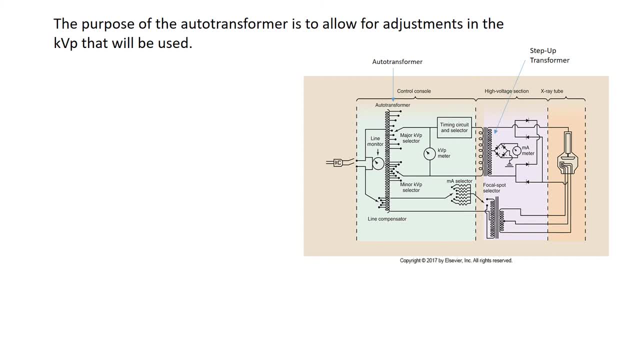 is a fixed number of coils so you have to vary the voltage before it gets into the step-up transformer. If you didn't all you could ever get if you were only feeding a single voltage at one level into the step-up transformer is a fixed number of coils So you have to vary the voltage. 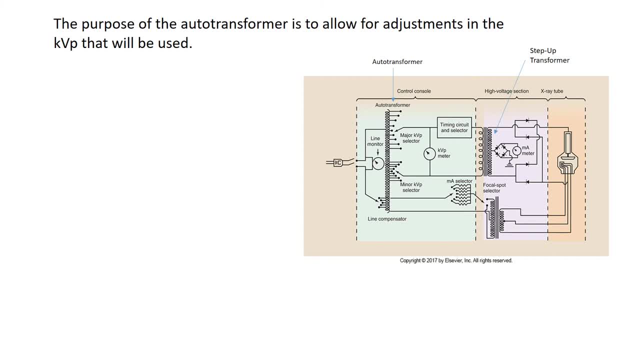 before it gets into the step-up transformer. You would only be able to get one kilovoltage setting and of course that would not be practical in radiography. Some of our kilovoltages we need to be high, some of our kilovoltages to be low, So we have to get that number of 220,. 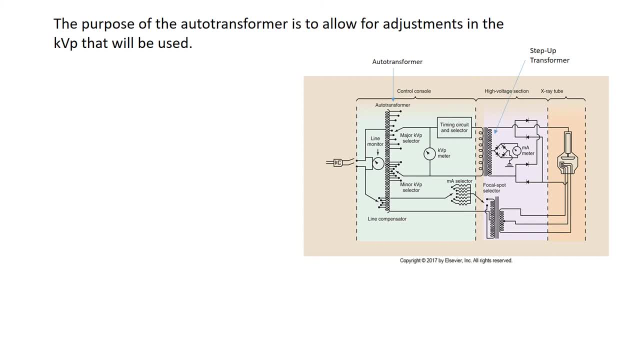 and we got to bring it up or down before it gets into the step-up transformer. So it says: notice that the electricity will eventually flow into the step-up transformer. The step-up transformer has a fixed number of primary coils and a fixed number of secondary coils. 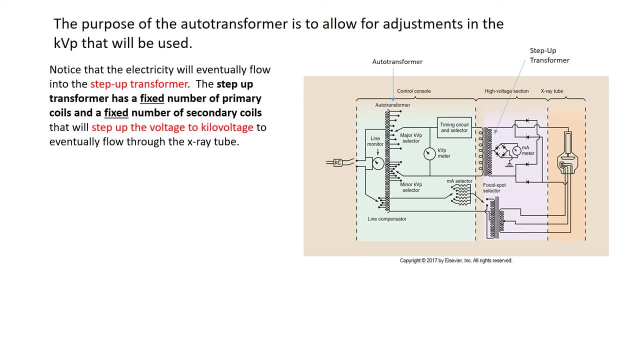 that will step up the voltage to kilovoltage to eventually flow through the X-ray tube. So if you kind of follow through on the drawing of the circuit there, you're going to see that eventually that kilovoltage now that is created in the step-up. 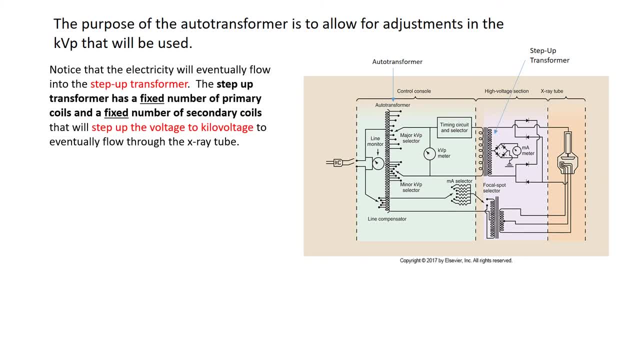 transformer is going to be filled with the X-ray tube And that's going to be the starting voltage fed into the X-ray tube, which is at the far right, As I mentioned, to vary the eventual kilovoltage flowing in the tube, the incoming electrical 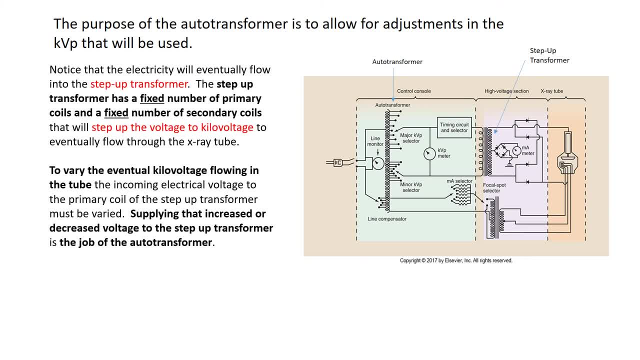 voltage to the primary coil of the step-up transformer has to be varied, Supplying that increased or decreased voltage to the step-up transformer is the job of the auto transformer. Some older X-ray consoles allow the technologist to vary the kilovoltages by tens and ones. 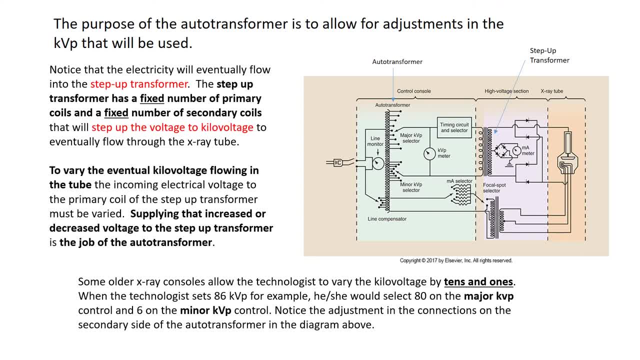 So, for example, on an older piece of equipment, if you're going to set up 86 kVp, you would have to select 80 and then you'd have to select 6. It would be two different dials, And the reason for this is that if we look at the drawing, you can see that you've got 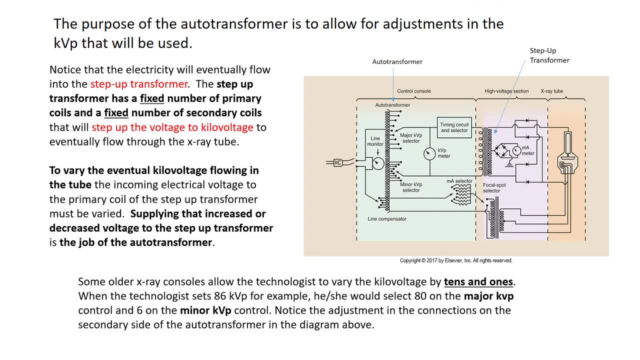 major kVp and minor kVp selectors. Your major kVp selector is going to be selecting in increments of 10.. Your minor kVp selector is going to be in increments of 1.. So on an older piece of equipment, you'd have to set up 80.. 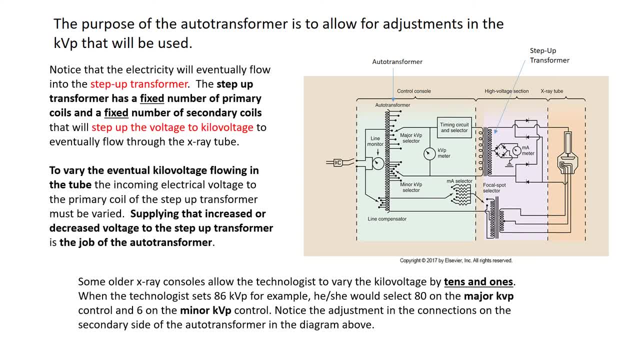 That's going to be the major caps on the auto transformer, And then 6,, which would be your minor caps on the auto transformer. Notice the adjustment in the kVp selector. You can see the connections on the secondary side of the auto transformer in the diagram. 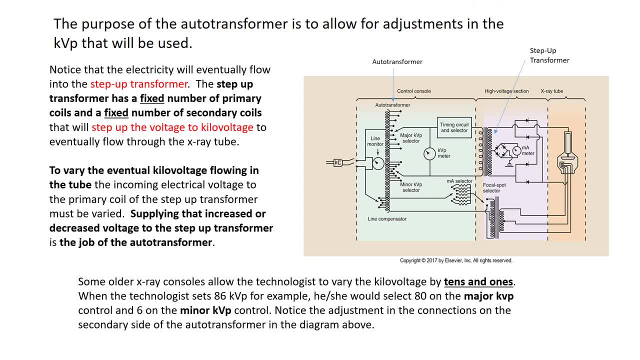 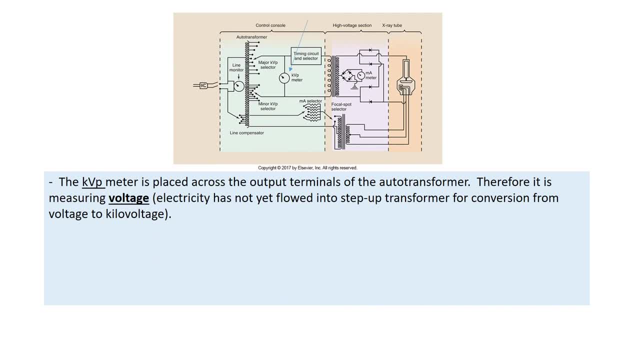 above. So you've got major kVp, minor kVp, selector taps. Now when we look at the drawing, so let's go back. What do we have? first, We've got the incoming power source. Of course, we've got to adjust it. 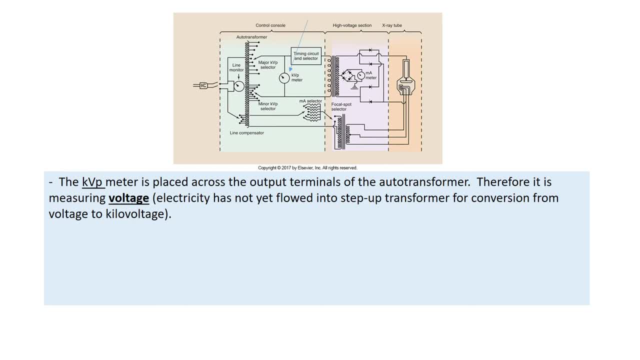 So that's going to be our line compensator, And then that 200 kVp, So that 220 volts. now that we have precisely at that level, we've got to bring it up or bring it down, And that's the job of the auto transformer. 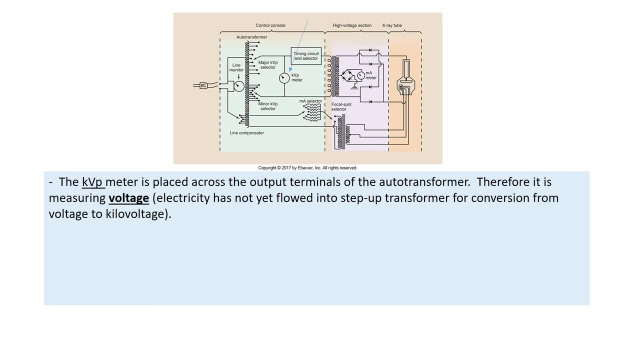 Now what did we say? We said that everything on your control panel has to be at low voltage. There is a kVp meter on your control panel. You know what kilovoltage you are setting. I want you to look at the position of the kVp. 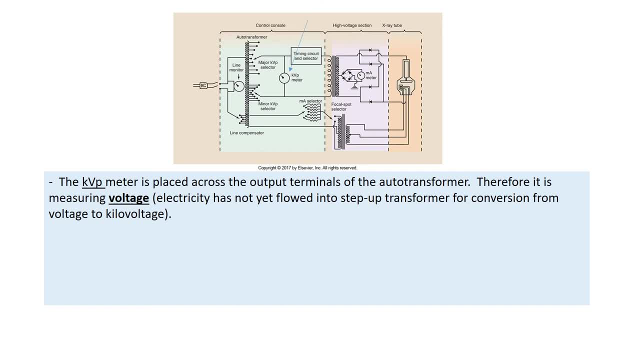 The kVp meter is going to be between the auto transformer, which is low voltage, and the step up transformer. Now, what's the job of the step up transformer? It's going to bring it from voltage to kilovoltage, So that's high voltage. 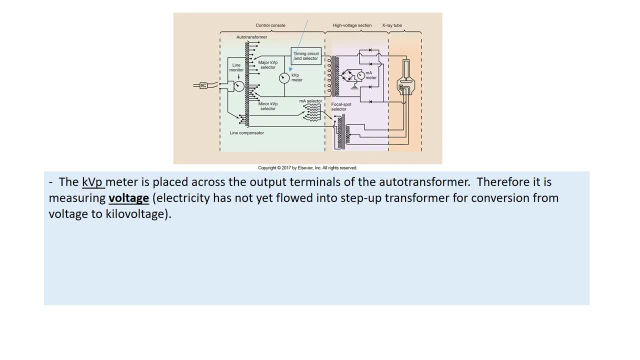 Since the kVp monitor or meter is on the control panel, It's going to be at low voltage On the control panel. it must be placed in the circuit in the low voltage section So we connect it in parallel across. we're bridging it across the circuit between the 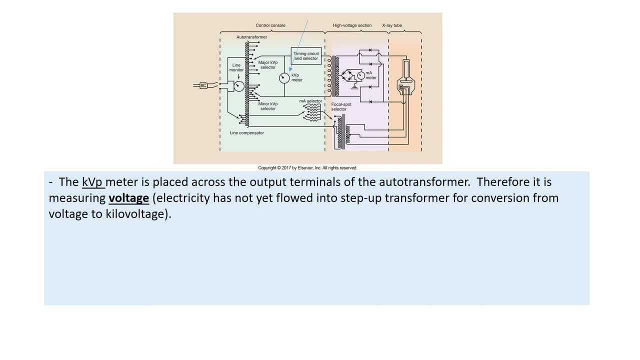 auto transformer and the step up transformer. What's interesting is that it's in the low voltage portion of the circuit- and it has to be because it's on the control panel, But it's actually going to measure the kVp. Now how can it measure the kVp if it's a meter? that's only measuring voltage. 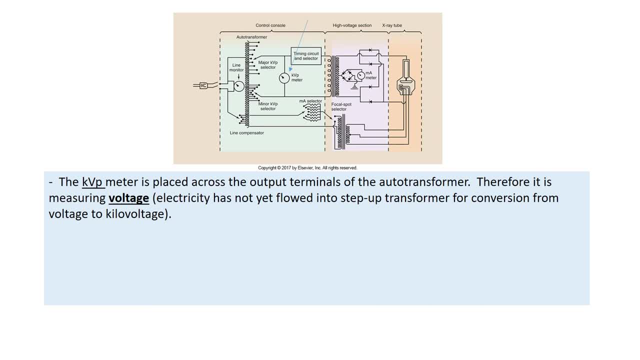 Well, the computer uses the transformer law and it knows how much voltage is going to be going into the step up transformer, which has a fixed number of coils, So whatever that voltage that's going to be going in is at. and then you do the math, you're. 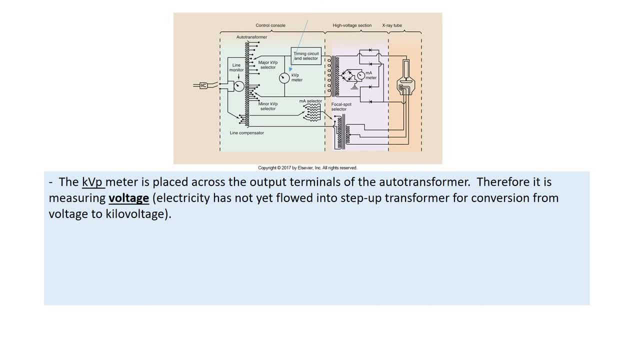 going to know what kilovoltage you're eventually going to end up with. So that's the kVp. So if we read, the kVp meter is placed across the output terminals of the auto transformer. Therefore it is measuring voltage. The electricity has not yet flowed into the step up transformer for conversion from voltage. 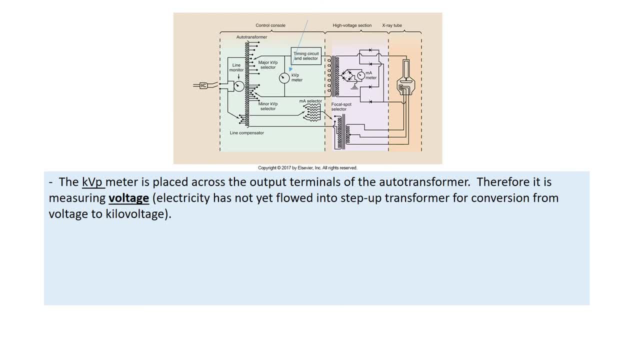 to kilovoltage. So that's often a question that you see on tests or on the registry. It's a little bit tricky, You would. you would think that the kilovoltage Meter, the kVp meter, is measuring kilovoltage, but it's not. it's measuring voltage. 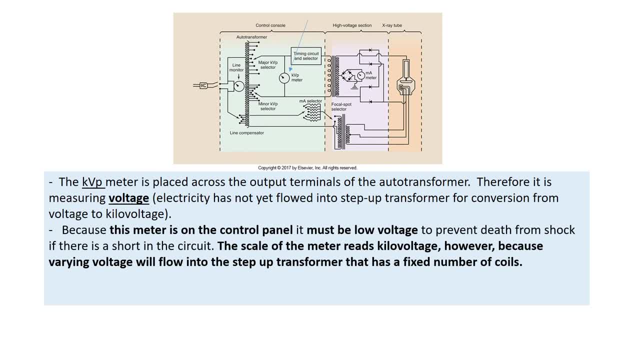 So, as I said, because this meter is on the control panel, it must be low voltage to prevent death from shock. if there is a short in the circuit, you don't want to be touching the control panel. and there's a short and now you're touching high voltage. 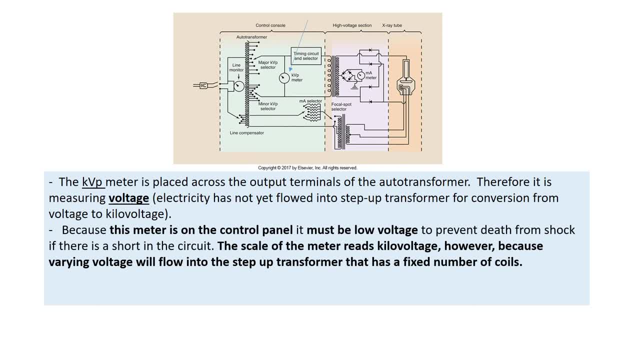 The scale of the meter reads kilovoltage. however, because the varying voltage will flow into the step up transformer. it's got a fixed number of coils. it's going to be able to calculate then the number of kilovoltage. So the scale of the meter reads kilovoltage. however, because varying voltage will flow, 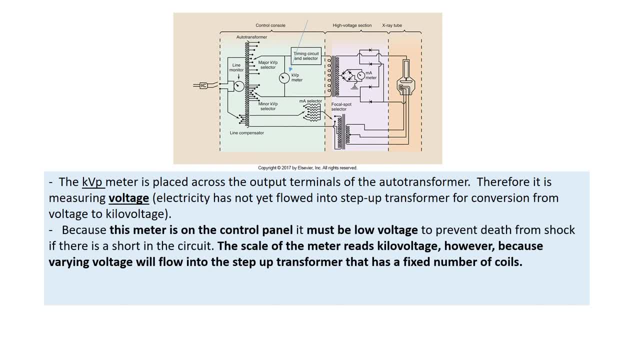 into the step up transformer that has a fixed number of coils. By applying the transformer law, math, the meter will be able to report the kilovoltage that will eventually flow into the transformer In the tube, even though it is only actually measuring voltage at that point. 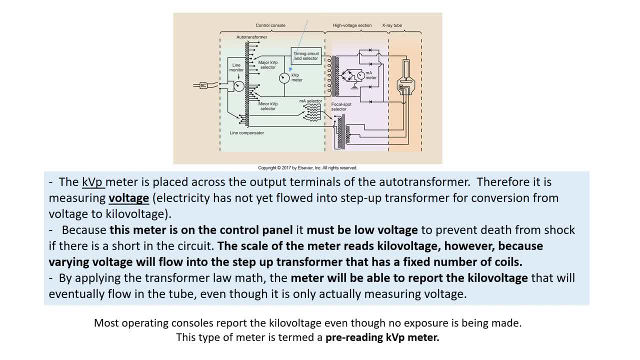 Most operating consoles report the kilovoltage, even though no exposure is being made, and there is a device called a pre-reading kVp meter that's incorporated into the circuit. You know what the kilovoltage is. when you go into the room, you can see it and it's, it's. 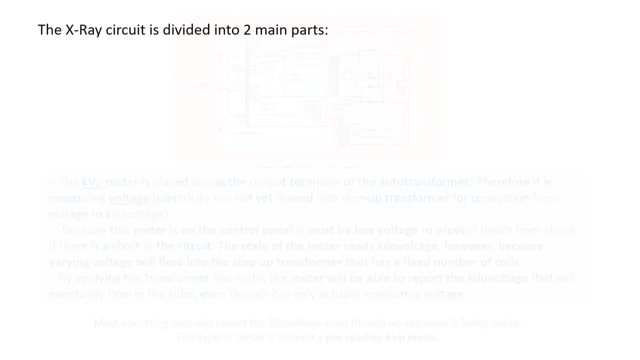 there it's set. The x-ray circuit is divided into two main parts. as I said, you've got the high voltage section. This is going to be used to generate the tube current, that amount of electricity, those electrons flowing from a cathode over to the anode. 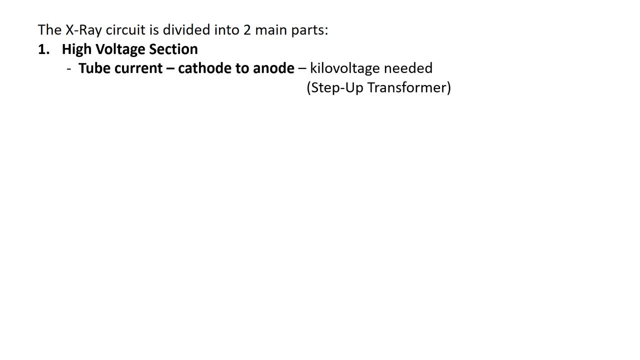 To do that, we're going to need kilovoltage, we're going to need a step up transformer And then, as I mentioned, we have a low voltage section. this is the filament part of the circuit. To heat up the filament, We need low voltage. to create thermionic emission, we only need about 10 to 12 volts, so think. 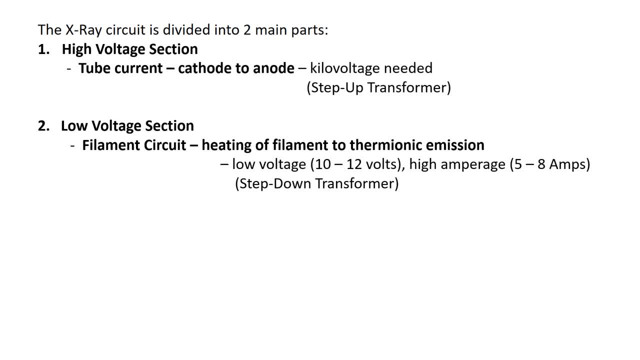 about it, you had 220 volts coming in. we got to bring down that voltage to 10 to 12 volts. But remember, when you bring down the voltage you bring up the amperage. So to heat up the filament to thermionic emission it needs low voltage, only about 10 to 12 volts. 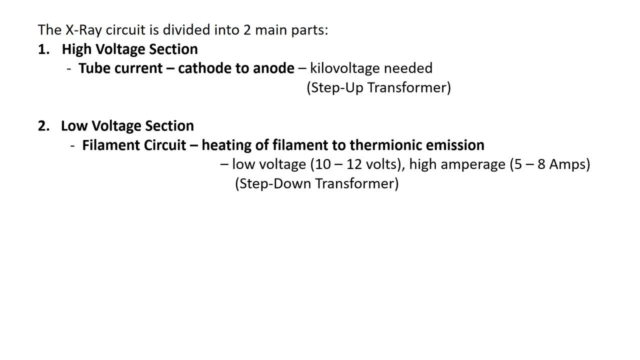 but you need really high amperage. Now I know the numbers. five to eight don't sound large, But one amp is a lot of electrons flowing through a circuit. So five to eight amps, you've got a lot of current, a lot of electrons flowing. 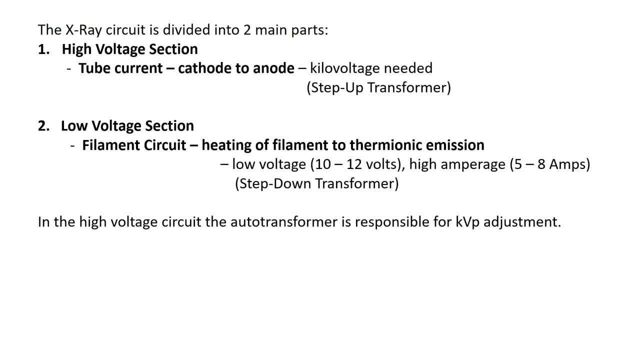 In the high voltage circuit, the auto transformer is responsible for the KVP adjustment And in the low voltage circuit, the filament circuit. There is another device that's going to allow you to change your MA values. that's called the rheostat or the MA selector. 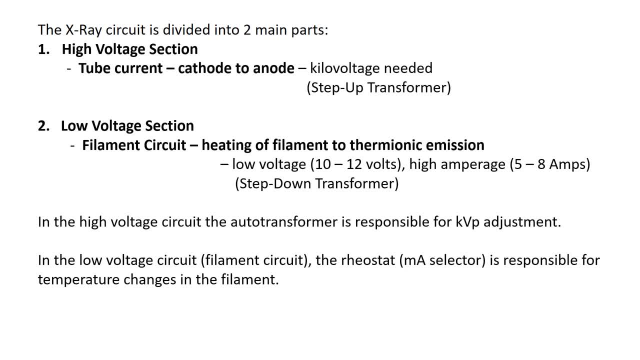 Basically what the rheostat or the MA selector is is. it's a variable resistor. you can either put more or less resistance on that electricity. that's eventually going to change the temperature of the filament, Which of course the filament is responsible for doing what. 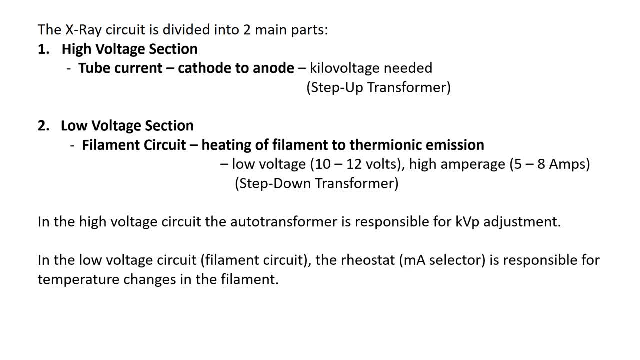 For boiling off electrons. The hotter the filament is, the more electrons are going to be boiled off. The cooler the temperature of the filament is, the less electrons are going to be boiled off. So what do we do when we take an x-ray? 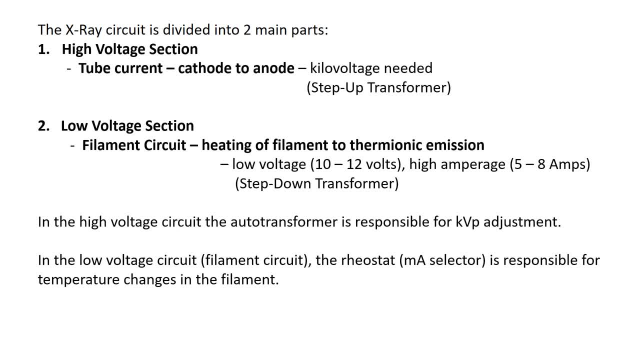 We adjust the kilovoltage- Now we know that that's really going to be part of the job of the electronics- a transformer- and we're going to adjust the ma values. this is the job of the rheostat, or the ma selector, as i mentioned. hotter filament: more electrons are boiled off, greater thermionic. 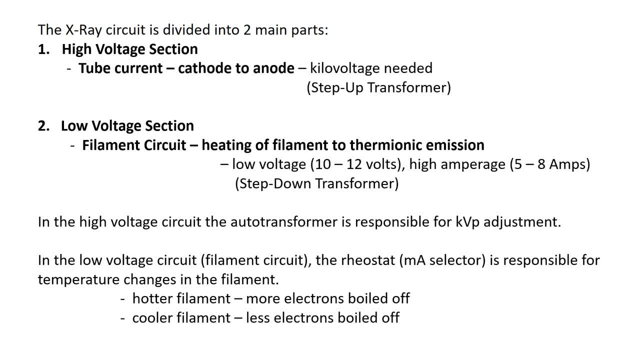 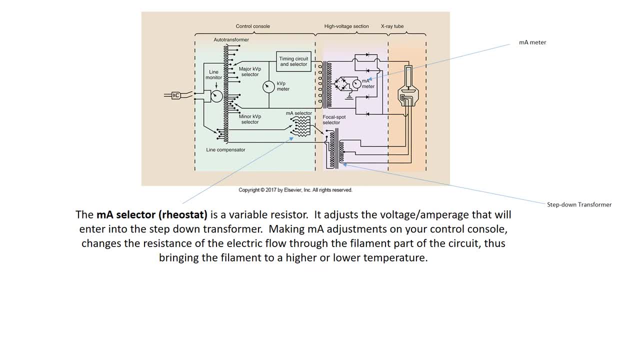 emission, cooler filament, less electrons are boiled off. so where is this ma selector or rheostat? so in our drawing, which this drawing is complementary of buchang is in your book, when we look at the top part of the circuit. okay, so we've got the incoming power source. on the left, the auto. 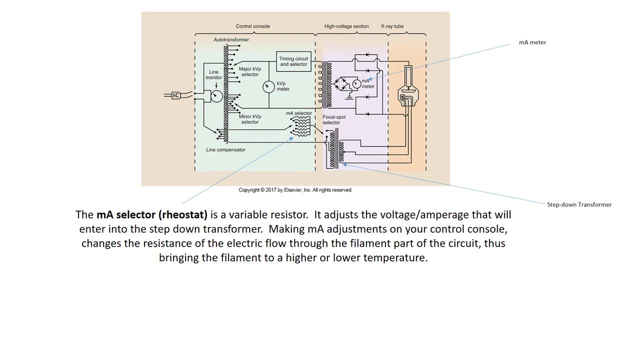 transformer. we know where the step up transformer is and we've learned that there's a kvp meter between the auto transformer and the step up. if we look to the bottom part of the circuit, here it's identified. i've drawn it with an arrow to show you. this is the ma selector, or rheostat. 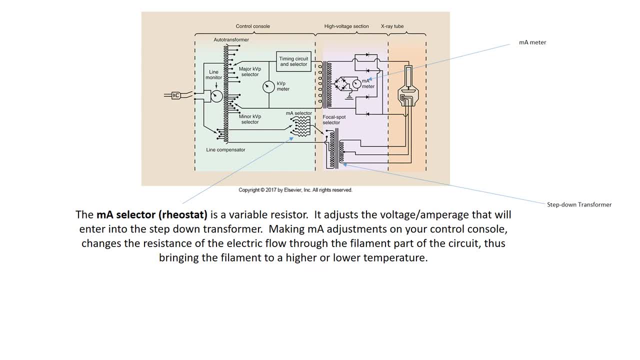 this is what is going to allow for changes in ma. so when you go from 100 to 300 to 1200 ma, this is the device that's going to be allowing for that selection to be made. that's the amount of electricity now that's going to be fed into the step down transformer, which also 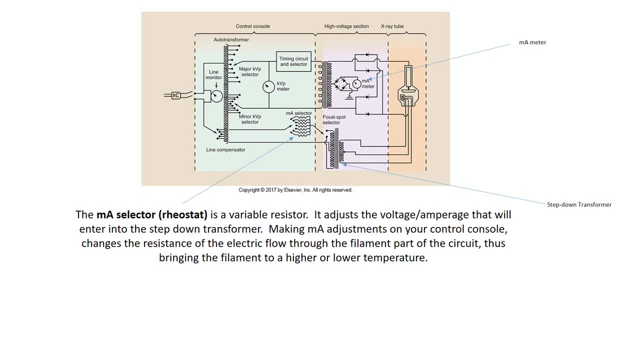 has a fixed number of coils. so it says the ma selector rheostat is a variable resistor. it adjusts the voltage or amperage. i should voltage and amperage. that will enter into the step down transformer. making ma adjustments on your control console changes the resistance. 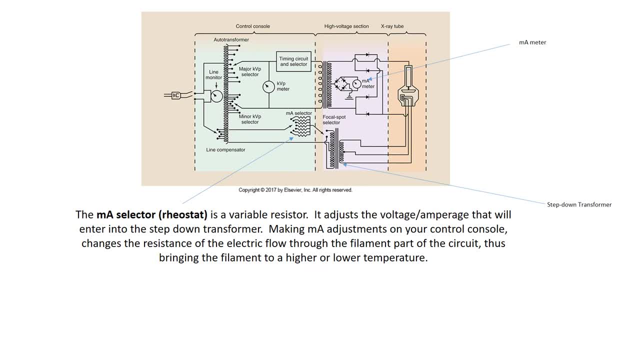 of the electric flow through the filament part of the circuit, thus bringing the filament to a higher or to a lower temperature. the x-ray tube current is monitored, just like your kvp was monitored with what's called an ma meter. now where is the ma meter? this is interesting. 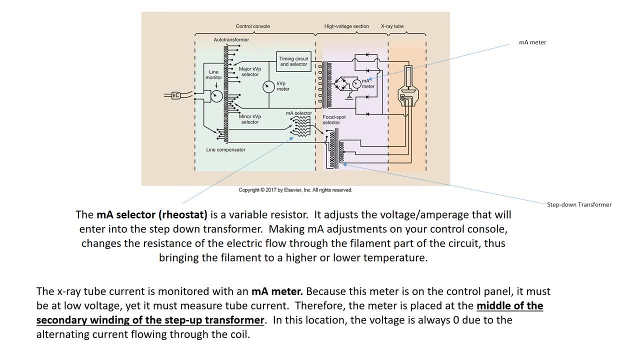 because the ma selector is in the filament part of the circuit. but the ma meter is actually- look at the drawing here- connected to the middle of the secondary winding of the step up transformer. why is it there? well, this is a meter that is on your control panel. 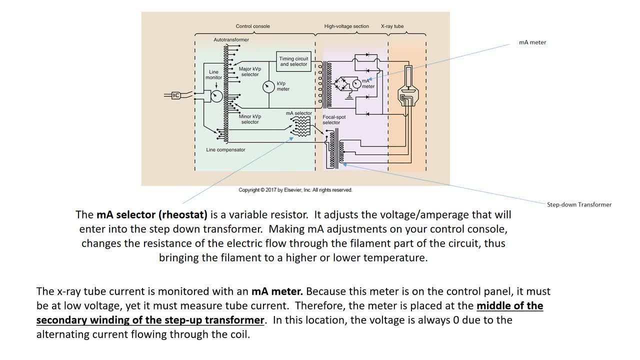 but it has to measure the amount of electrons that are eventually going to flow across the gap between the cathode or where the anode. we've got to make sure, because that meter is on the control console, that it is low voltage. but you're saying, wait a minute, it's in the high voltage section, but the position of where it 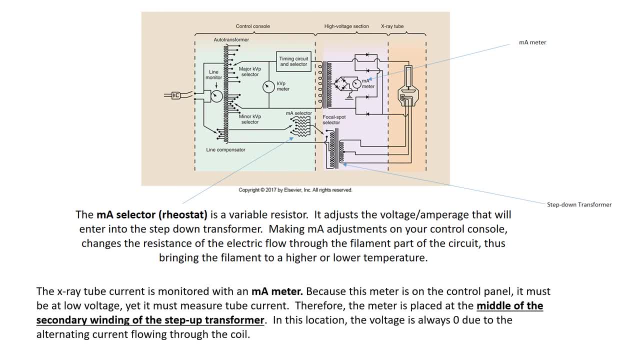 is connected becomes very significant if we read what it says here. because the meter is on the control panel, it must be at low voltage, yet it must measure tube current, the number of electrons flowing from the cathode to the anode. therefore, the meter is placed at the middle of the secondary 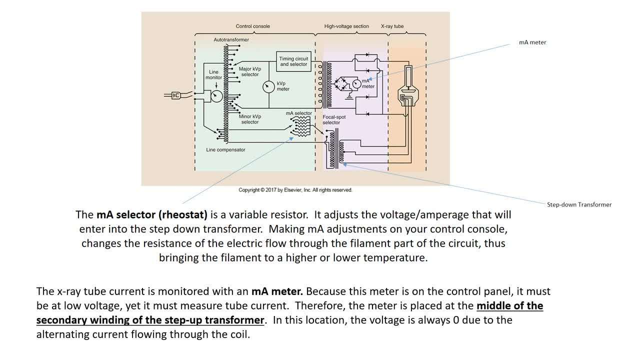 winding of the step-up transformer in this location and only at that location. on that coil the voltage is always zero due to the alternating current flowing through the coil, and we'll get more into that when we talk about the step-up transformer. but in that position right now i